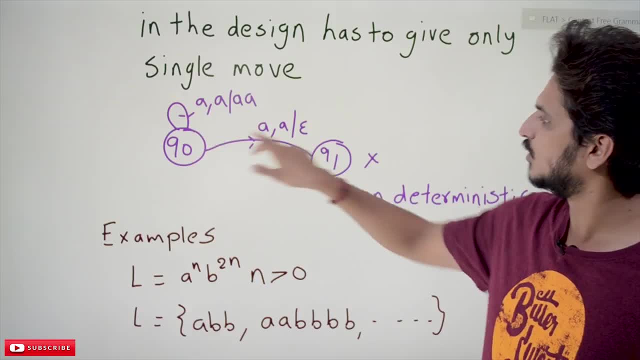 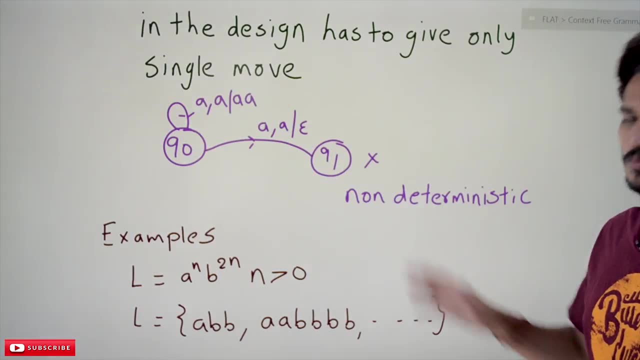 Second, A is the stack symbol For the same A, comma A. we are moving to Q1. also, We are taking two moves. This is not deterministic finite automata- pushdown automata. It is not deterministic finite automata. We call it as a non-deterministic finite automata. 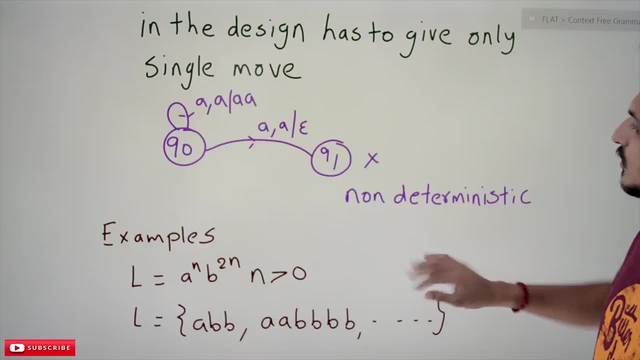 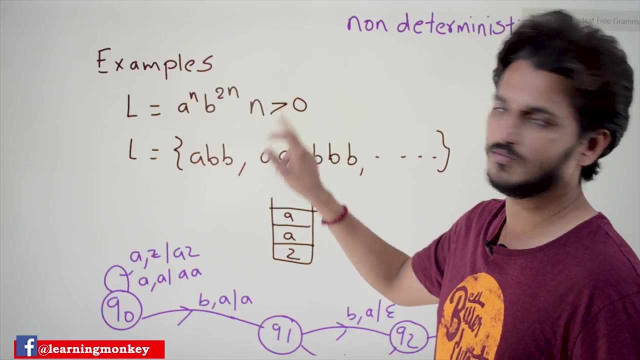 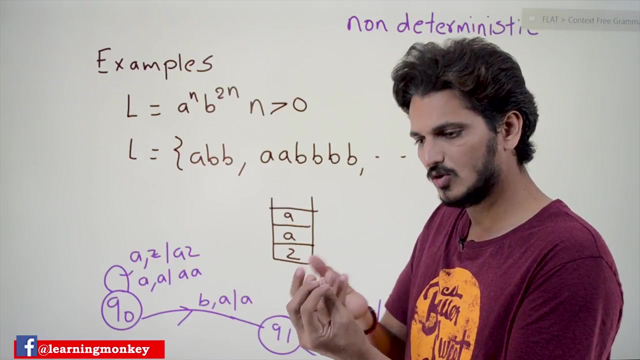 So, coming to the examples, we do some practice examples how to write the pushdown automata for a given language. Take: L is equal to A power and B power 2N, where N greater than 0.. When N is equal to 1, A, B. B means A's followed by B's. If you have single A, you 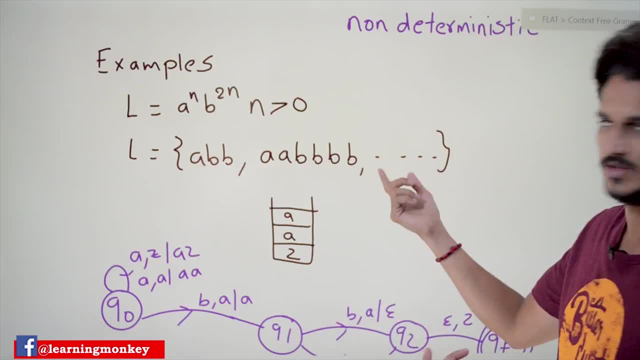 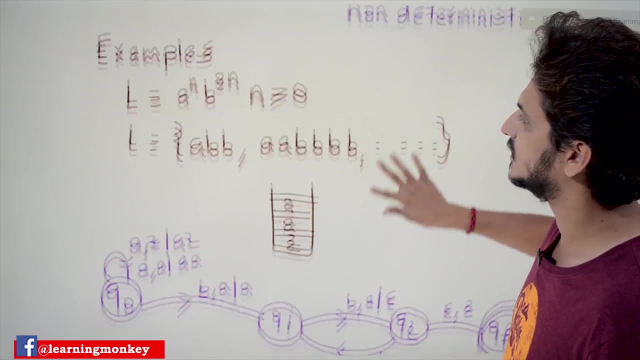 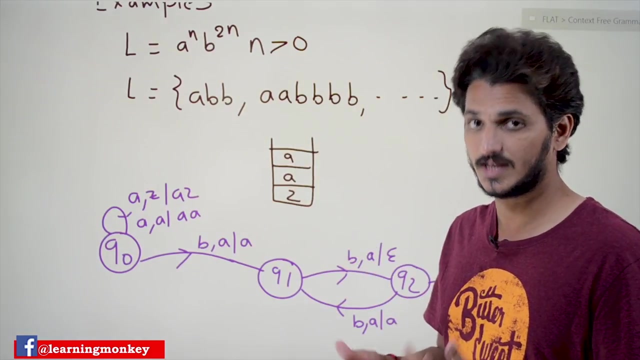 have to take two B's. If you have two A's, you have to take four B's, Multiples of two. that is how you have to identify the strings. So what we have to do for this: Whenever you see A push on to the stack. So take a stack In our pushdown automata we are 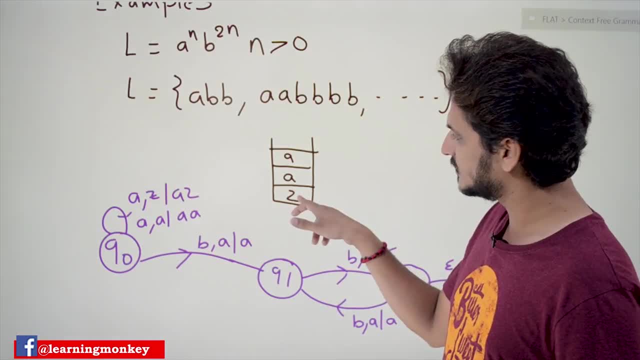 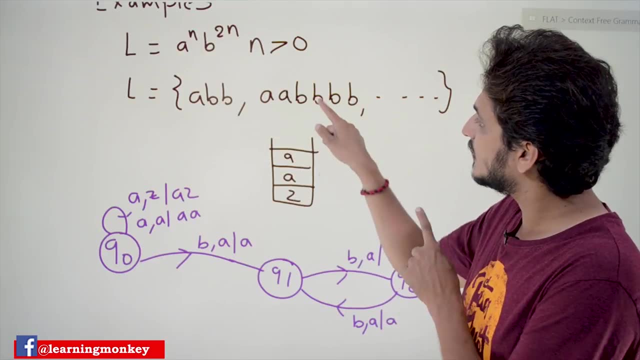 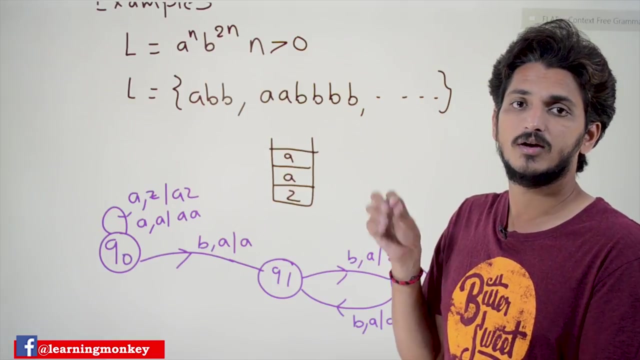 having a stack. memory space On the stack top is Z initially. If you see A, push on to the stack. If you see another A, push on to the stack. Whenever you see two B's, pop one A. Whenever you see next two B's, pop one A. For every second B you have to pop. 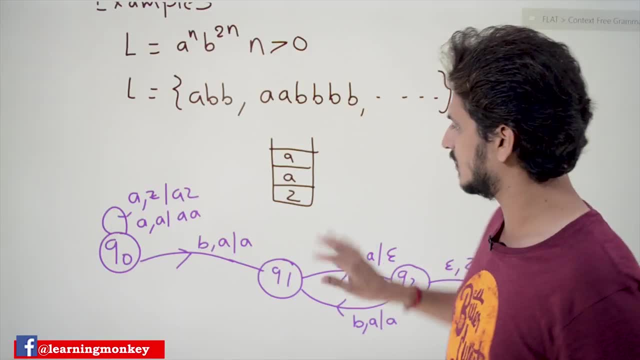 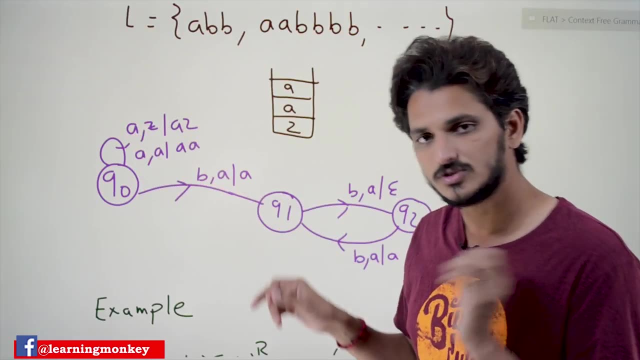 the A. That is what the logic is, How to write the logic. We are starting from Q0.. On Q0, if you see the input symbol is A and stack top is Z. yes, you have to push the A. That is why A- Z, If the input symbol is A and the stack. 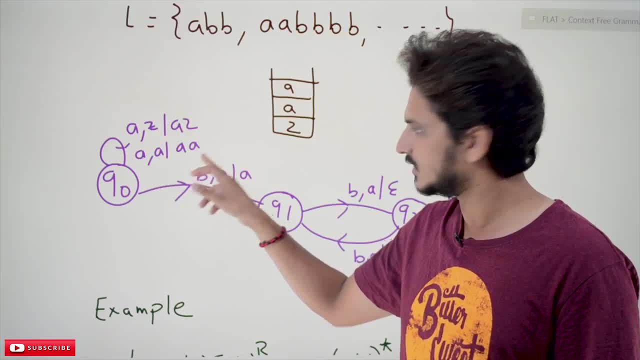 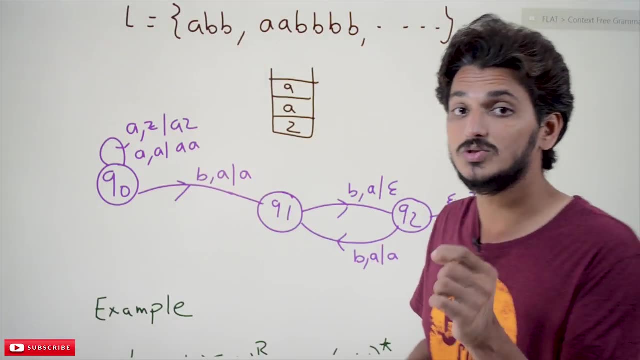 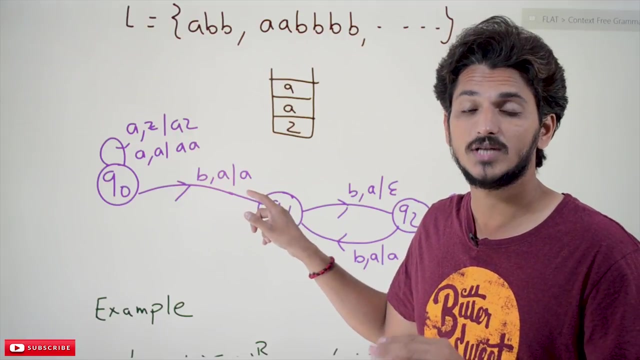 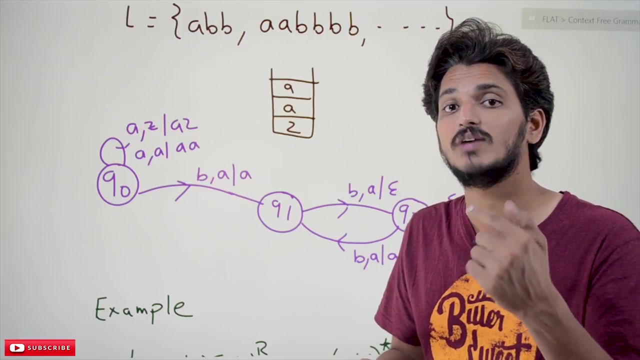 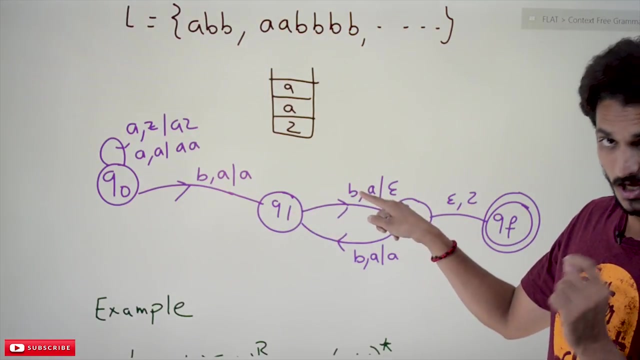 top is A: push on to the stack. So that is why, if you do the push operation A, A is the output on the top of the stack. Whenever you see B, we have to take one step. Whenever you see B, we have to take one step. If you see, the input symbol is A and the stack top. 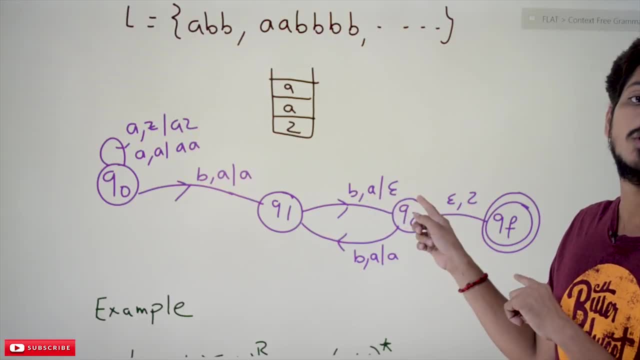 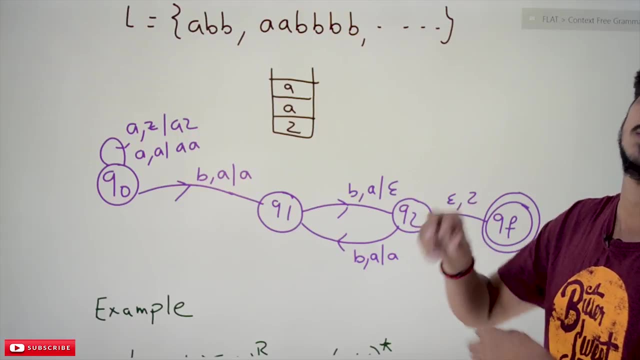 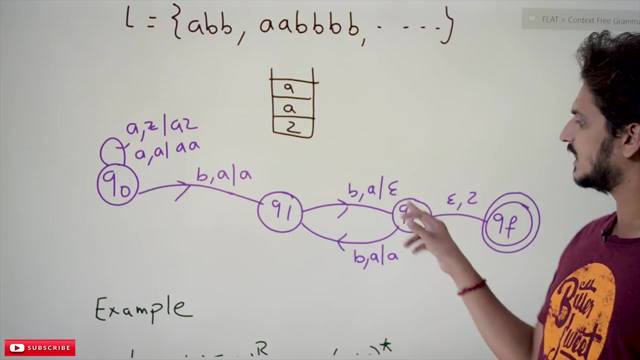 is B and stack top is A, we are doing pop operation. That is why, epsilon, So we had seen two B's For second B. we are taking action. We are taking action. We have to pop the symbol A After that. if you see one more A, move on to Q1.. Second B: pop B, B, B, B For every. 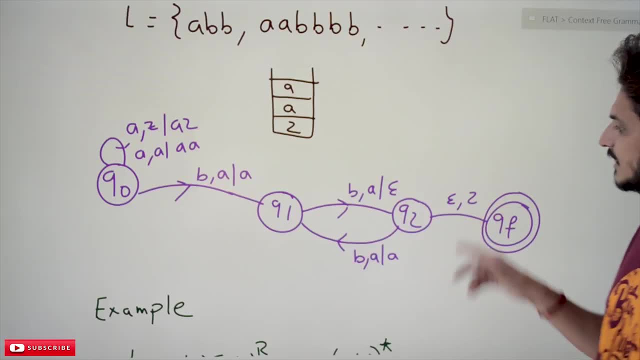 second B, pop one A from the stack And the stack after that. if you see, the input symbol is E- epsilon, and the stack top is Z. we are moving to final state. We have written the pushdown automata based on a final state logic. We are moving to final state. Coming to the 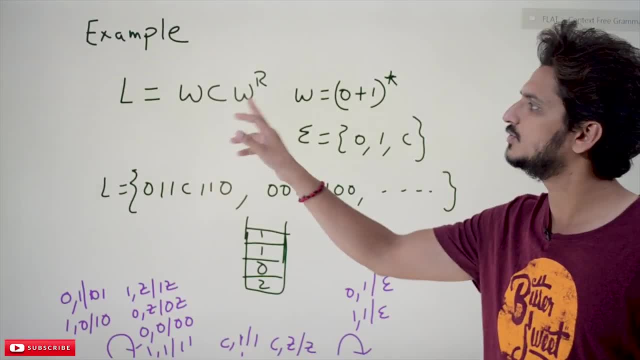 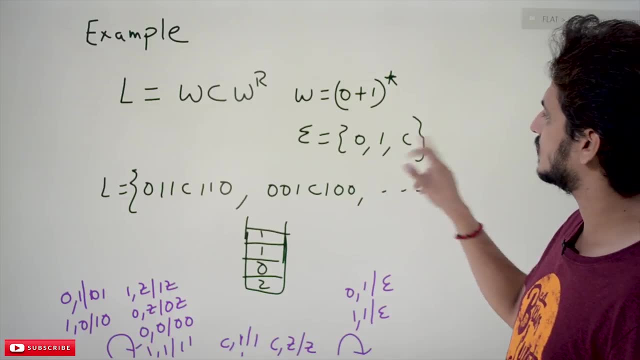 next example. We are taking one more example. L is equal to WCW power, R. What's the meaning of this language? W is equal to 0 or 1 whole star and sigma is equal to 0,, 1, C. The language consists: 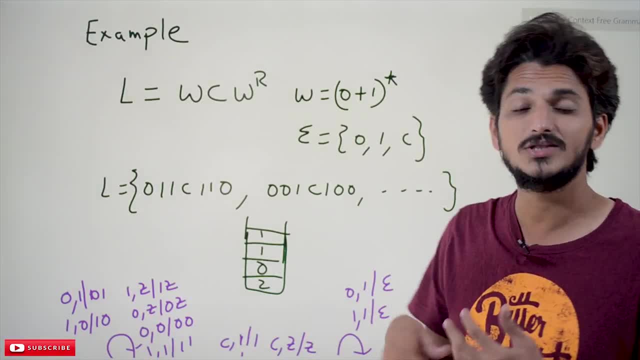 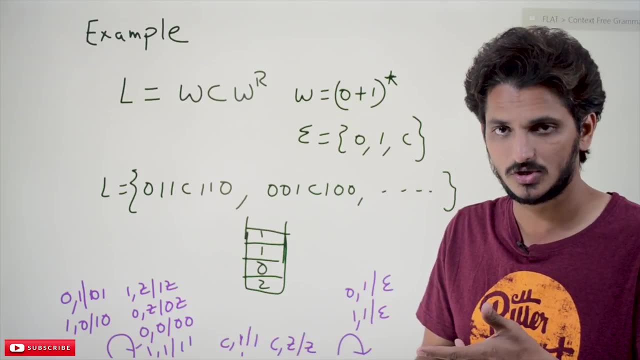 of strings. W means 0 or 1 whole star. It means you can write string that belongs to 0 and 1.. Any string you can write. You can take epsilon. You can take 0.. You can take 1.. You can take 0, 1.. You can take 1, 0.. Any string that is obtained by using 0 or 1 whole. 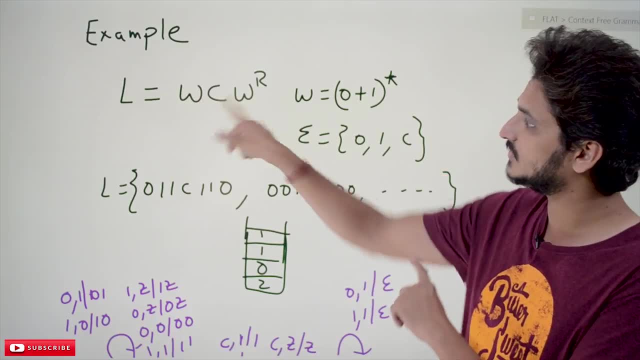 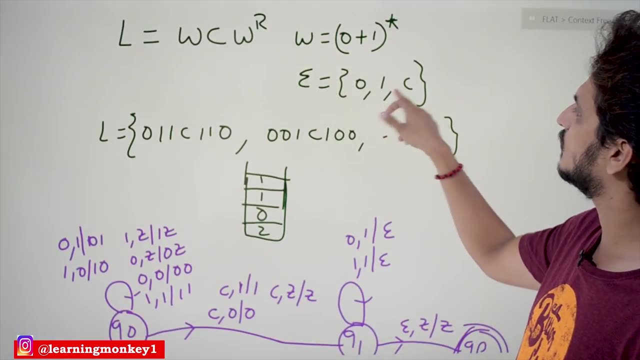 star, you can take this here Exactly. reverse of the string should be present here. That is what W power R means. What string So the input symbols are? sigma is equal to 0, 1.. C is also there in the input symbols, input alphabet. So C is there. The strings contains: 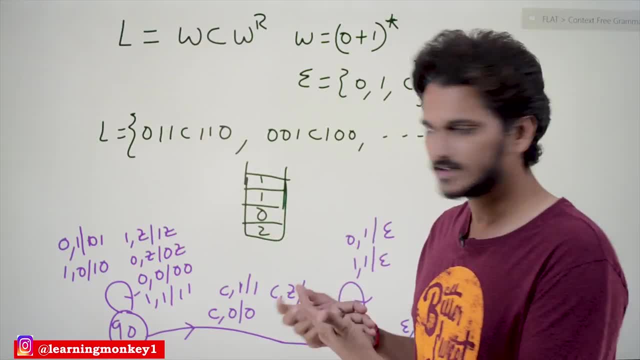 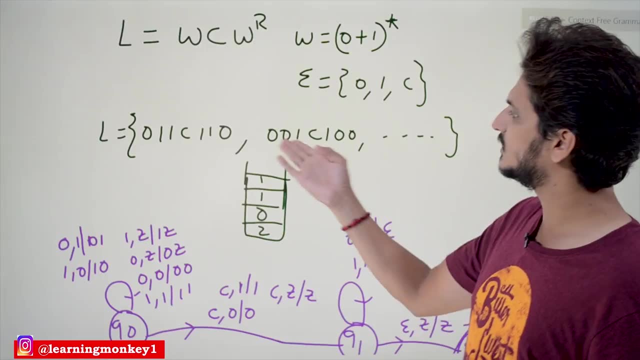 like this: 0, 1, 1, C. 1, 1, 0. This is exactly: 0, 1, 1.. What's the reverse of it? 1, 1, 0.. In between, we are having C. The same way: 0, 0, 1, C. Whenever you find C, 0, 1, 1, C. 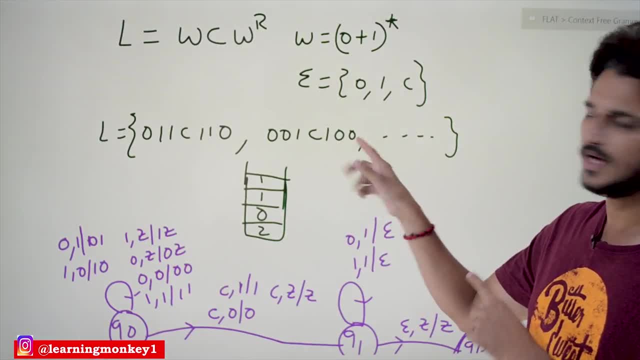 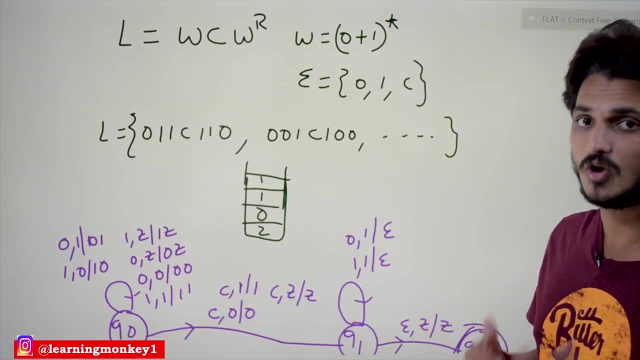 1, 0, C. after that, the string should be exactly reverse of this string: 1, 0, 0.. These type of things should be accepted. How to write a pushdown automata for this language Logic is very simple. So whenever 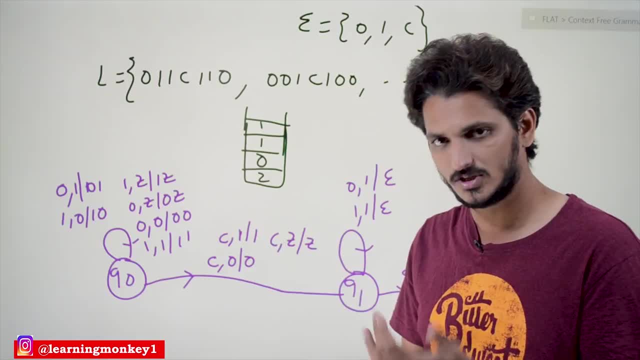 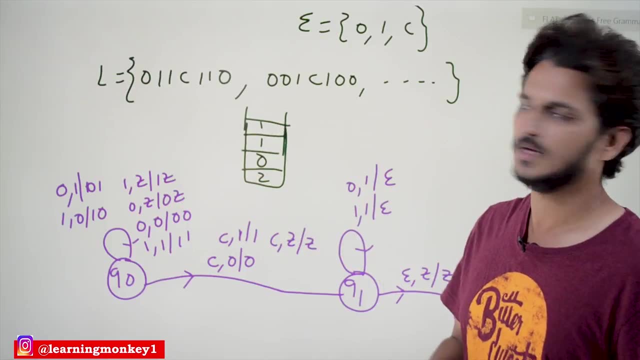 you find C. before that, whatever you observe, you find 0, you find 1, any number of 1, you find 0. Whatever you find before C, push onto the stack Great. So whenever you find 0,. 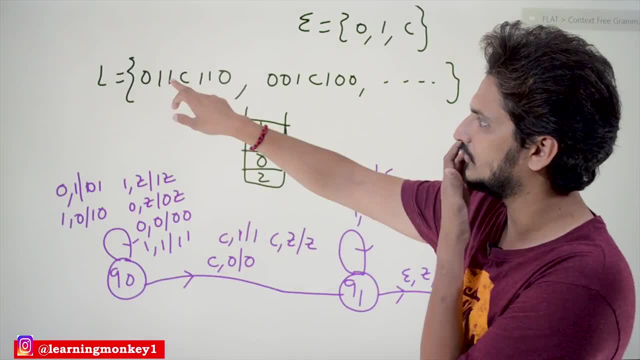 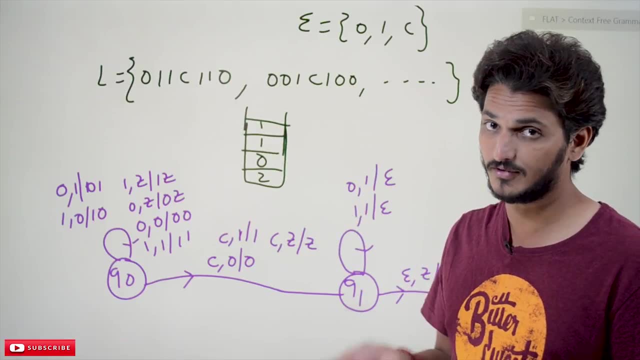 push onto the sticky Perfect Script finished. Thank you onto the stack. if you find one, push onto the stack. if you find one, push onto the stack whenever you find C. from there onwards logic should be different. after that you find one, this one should be matched to this one. then only we can say: 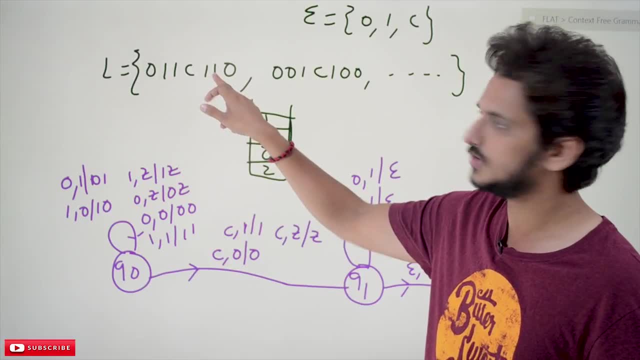 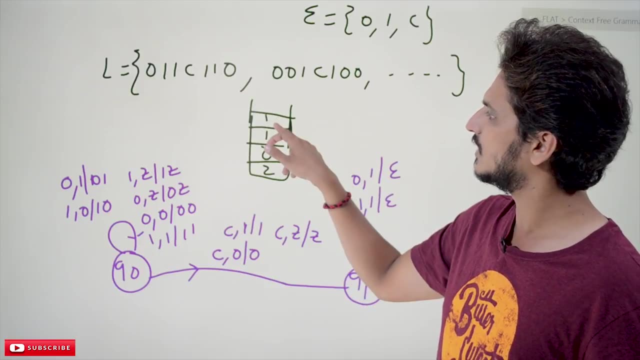 that it is reverse of the language. this one should be matched to this one. this one is top of the stack. this one is top of the stack if you find the input symbol is one. if the stack top is one pop, it means exactly. you are checking for the reverse of the. 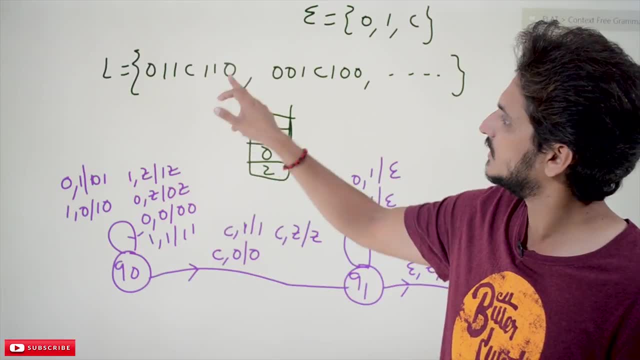 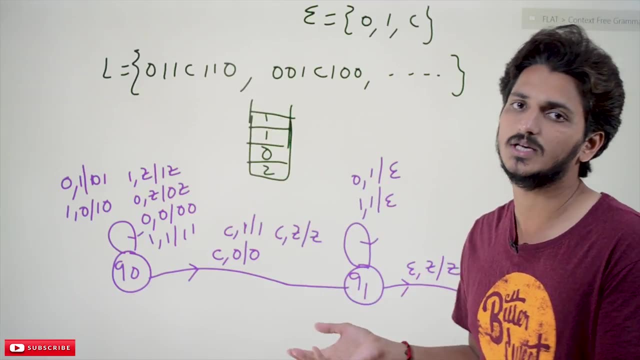 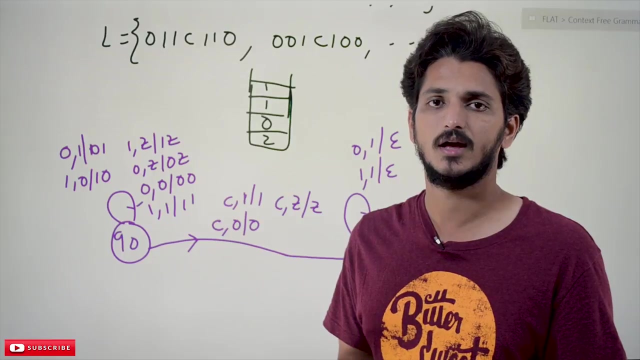 string. reverse of this w. the second one is one: stack top is one, pop it. the third one is zero. stack top is zero, pop it. this is what the logic is. it's very simple. so how to write the? we are starting from q, naught on q, naught, whatever you find, push on to the stack. and one important point: 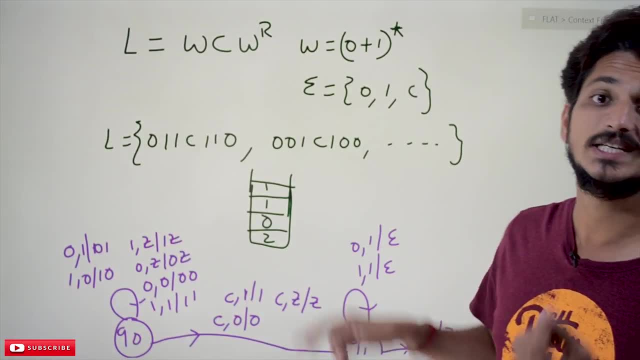 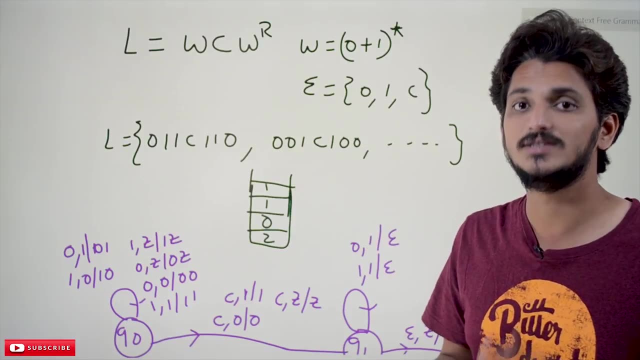 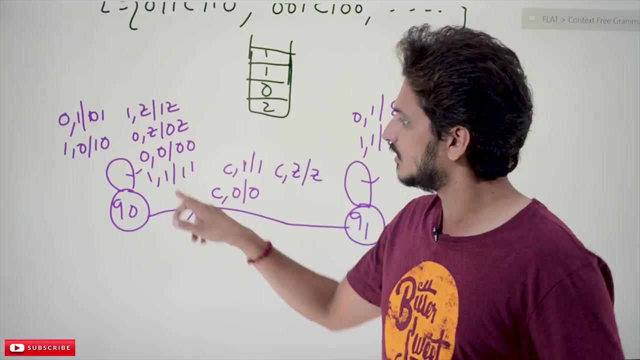 you have to understand here. it is going to accept single c also. zero or one whole star means this can take as epsilon. this can take as epsilon what's remaining in the string c. single c is also there. that logic also you have to incorporate into the pushdown automata. so if you see the one, if you 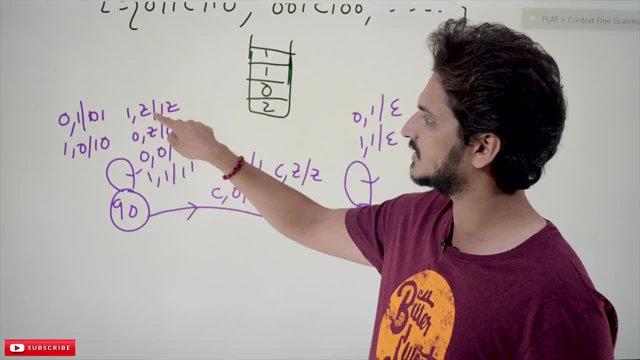 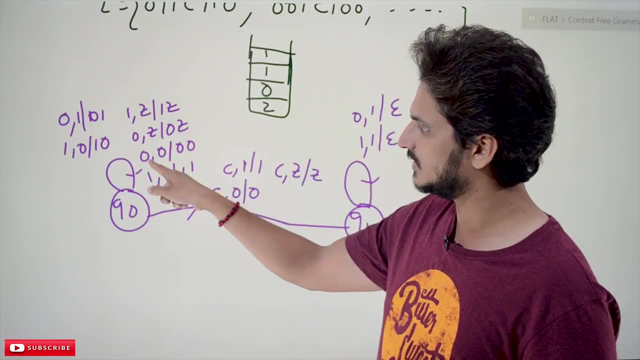 say how on q naught. if you see the input symbol is one and stack top is z push, one z. if you see the input symbol is zero, stack top is z push. if you see the input symbol is one and stack top is z push. if you see the input symbol is zero, stack top is z push. 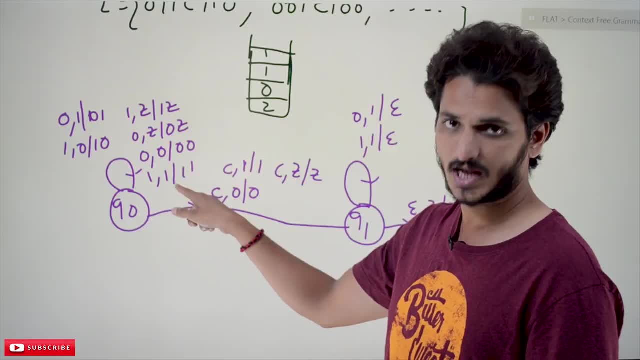 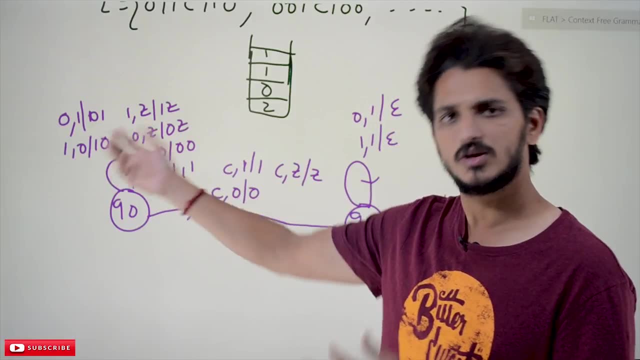 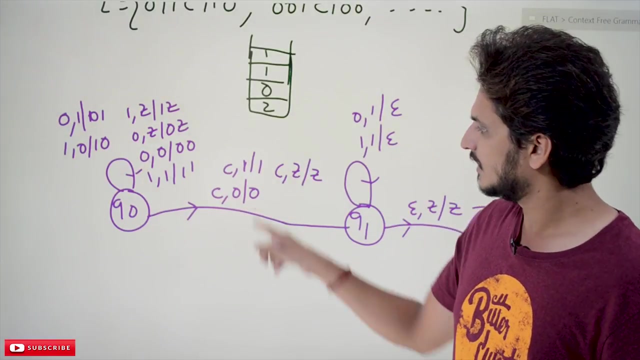 if you see the input symbol is one stack top is one push input symbol: zero stack top. one push input symbol: one stack top is zero, yes, push. all the possibilities has been written. whenever you find the input symbol is c and stack top is zero, we are leaving it as it is. we are not doing any. 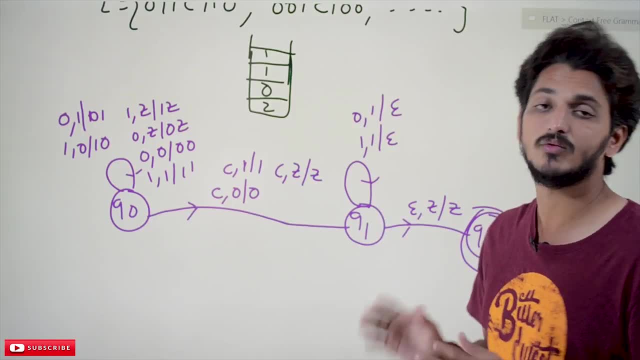 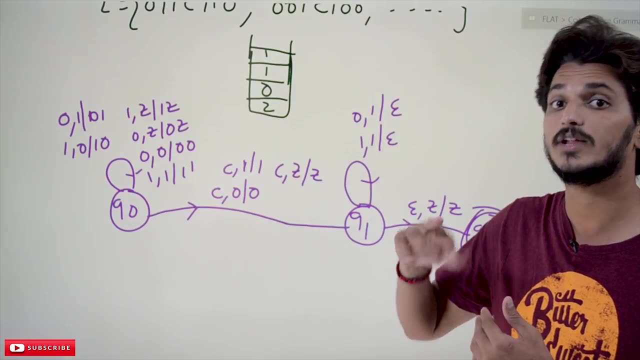 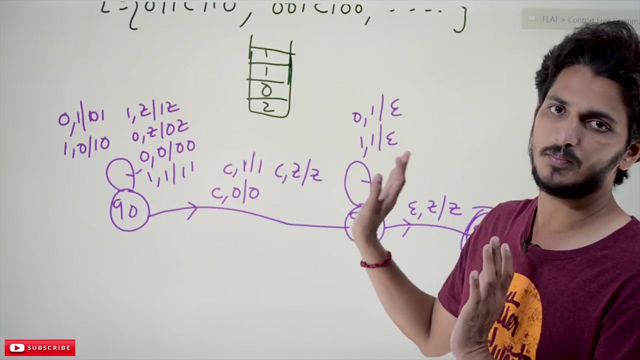 action, no operation. we are moving to q one. why we are moving to q one, then from next turn onwards we have to see for the, we have to check for different logic. we have to do the pop operation if the input symbol is c and the stack top is one. no operation if the input symbol is c and the 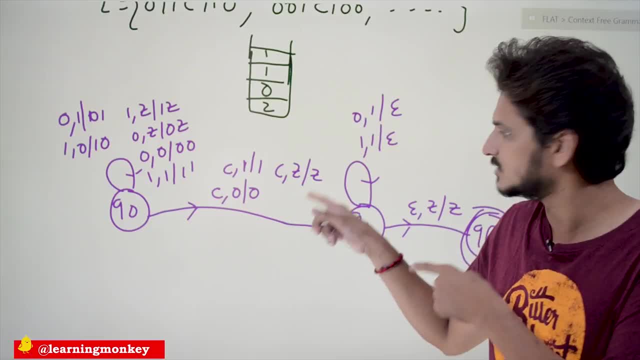 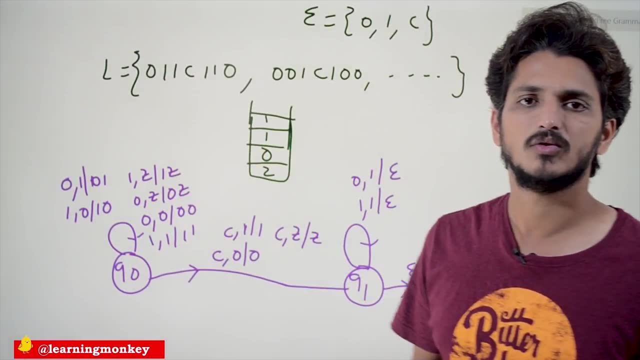 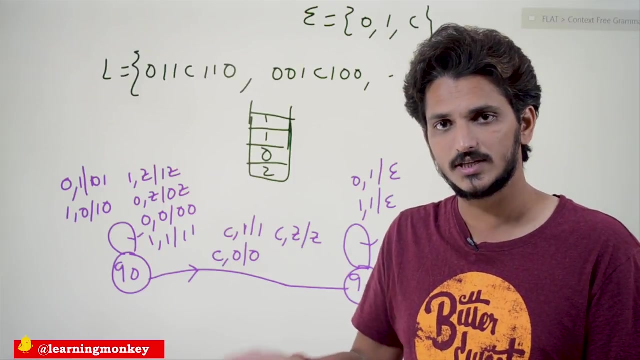 stack top is z: no operation, in which cases you will get this option. c. stack top is z: see here before c. if it is epsilon what you are going to identify, the first input symbol is c. we have to accept that. after c, if it is nothing is there. yes, we have to accept it. that's why we